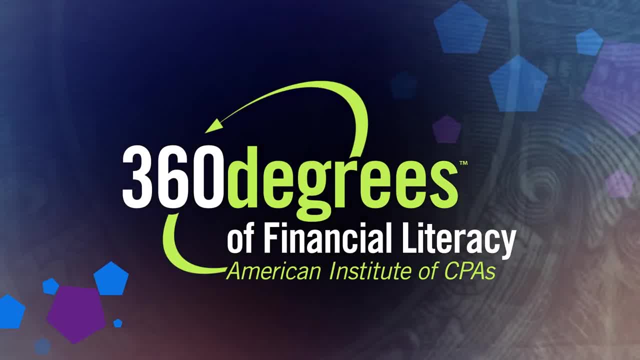 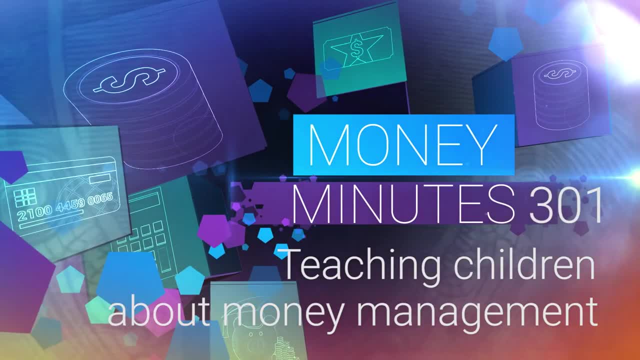 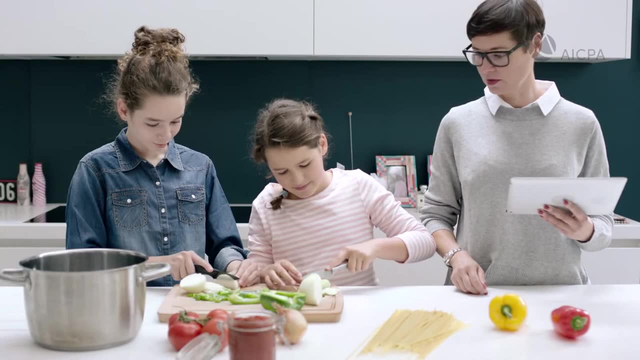 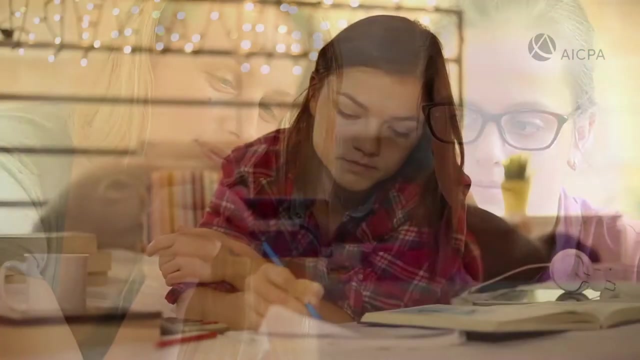 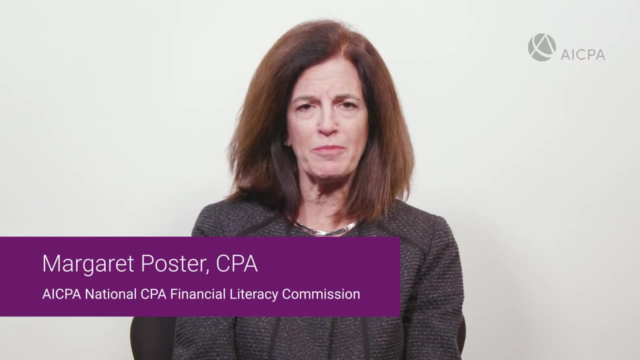 Parents are already focused on teaching good habits to their children, like how to be healthy and helpful to others. Managing money is one more habit where starting early helps. A strong financial knowledge will benefit a child their entire life. Hi, I'm Margaret Poster. CPA member. 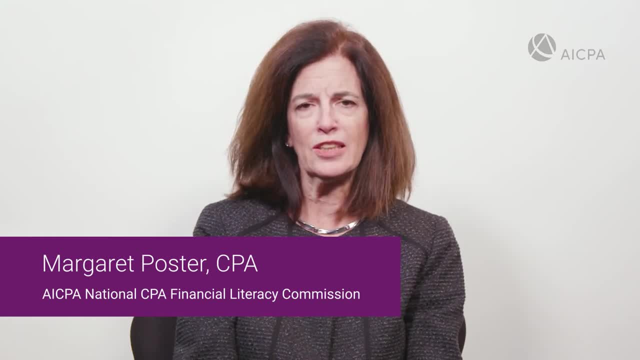 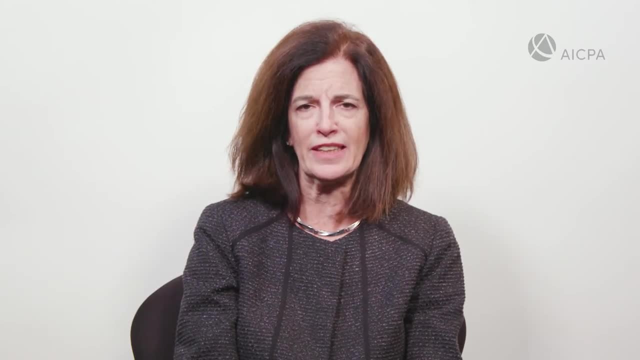 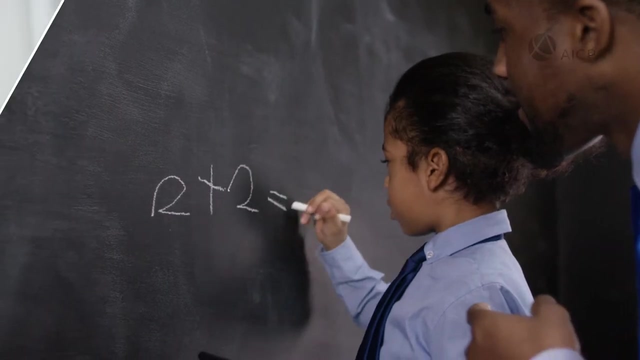 of the American Institute of CPAs National CPA Financial Literacy Commission, and here are a few ways parents can start teaching financial lessons at home. Teaching children about money is a big job and there are many ways to go about it. A good place to start is by encouraging your child to be 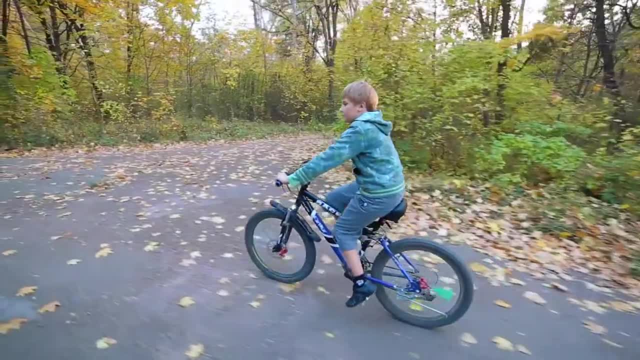 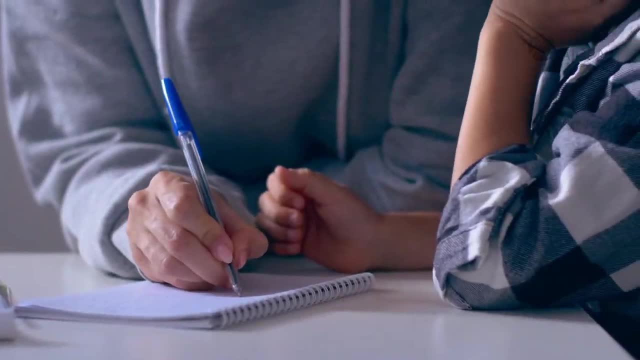 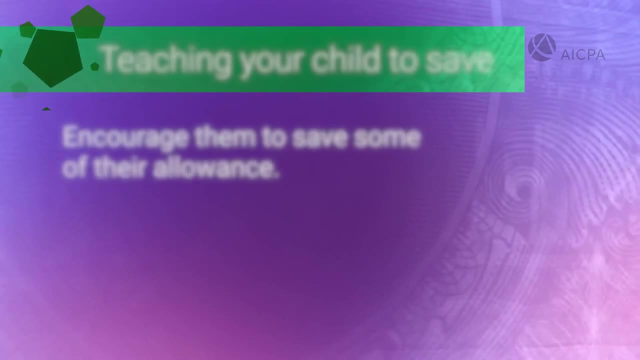 a better saver. So, for example, when a child wants a bigger purchase, such as a bicycle that costs $100, you can help them come up with a plan for how they're going to save enough to buy it and how long it will take If, for example, they receive an allowance of $30 a week and $10 of 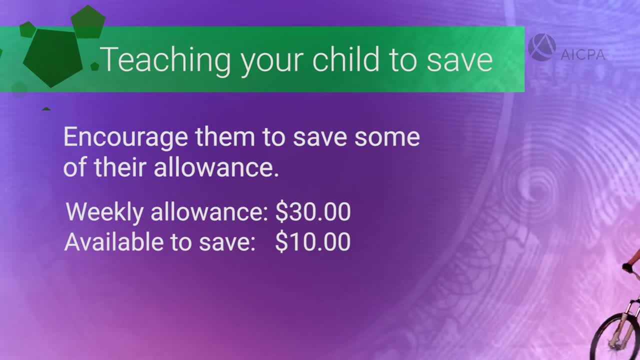 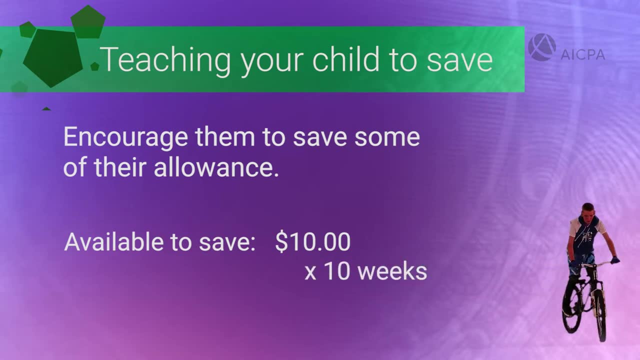 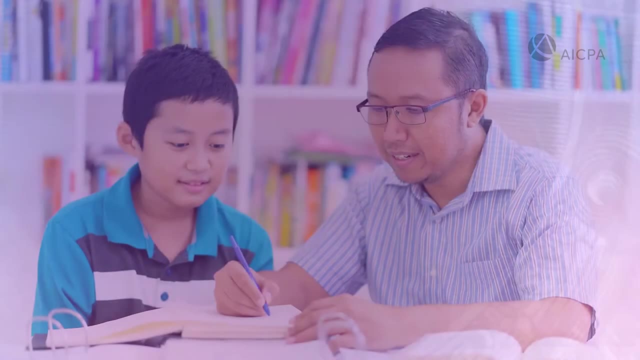 that amount is left over for discretionary items, they can save the $10 towards the purchase of that bike. It will take them 10 weeks to have the $100 they need, which may seem like a long time, But you can do things along the way to help keep track of their progress, like creating a chart and marking. 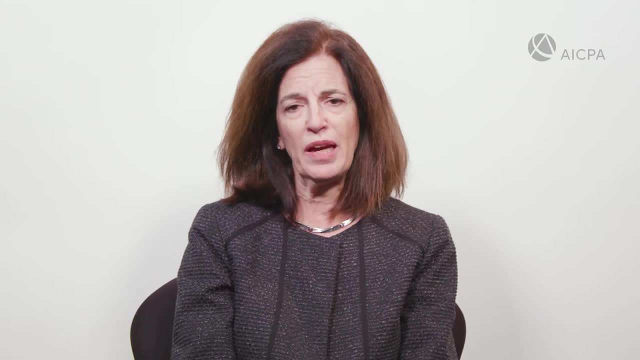 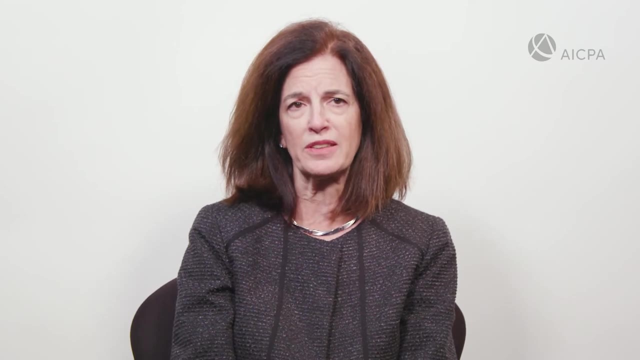 off how much has been accumulated to date. As they make progress towards the goal, you can discuss which bike to purchase and understand the pros and cons of different models. As they get closer, you can talk about where they'll use it and who they'll use it with By focusing. 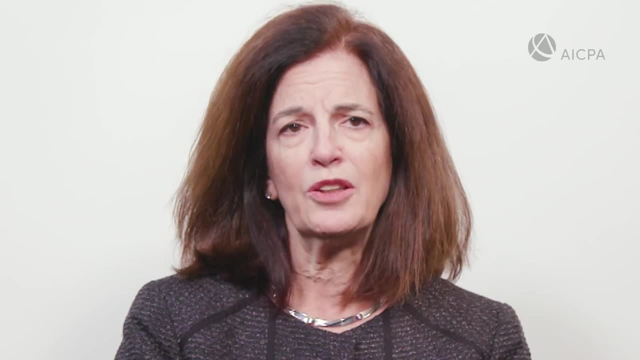 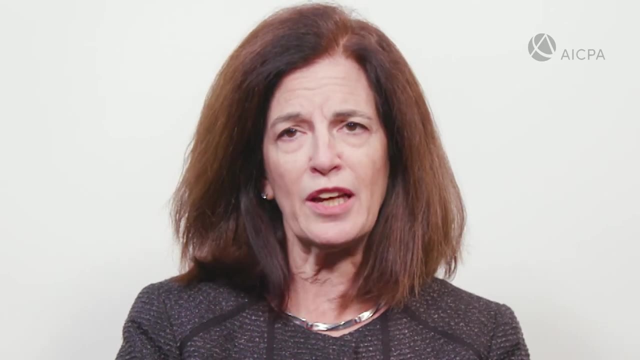 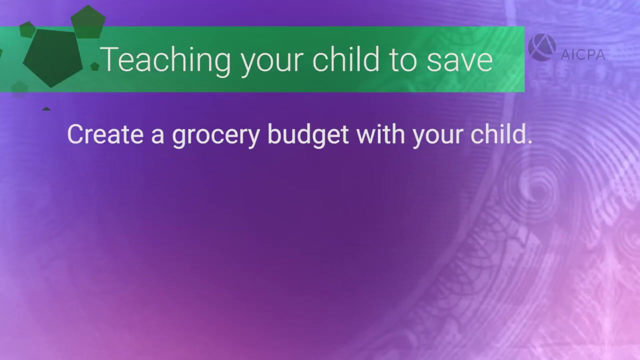 on different aspects of actually owning the bike. you will help build an understanding of the value of the purchase and excitement towards actually owning it. There are many opportunities that can be turned into money management. teachable moments Before buying groceries. create a budget with your 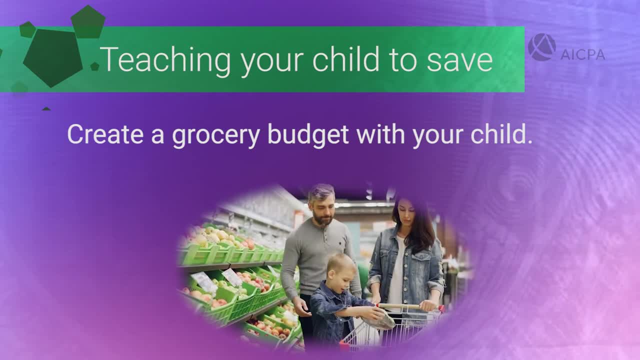 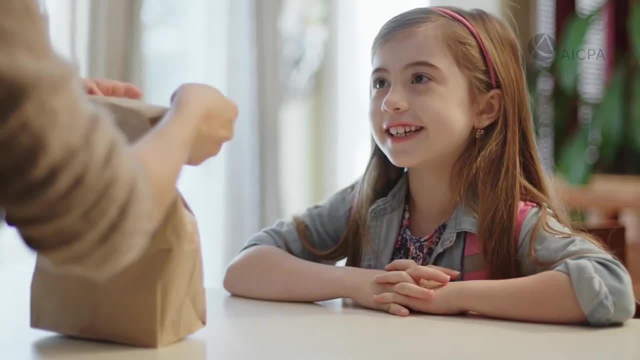 child, You can talk about the staple items the family needs for healthy eating and, where possible, you can give children a choice about what items to include for their school lunch. And then, within the shopping center, you can talk about the items the family needs for school lunch And then, within